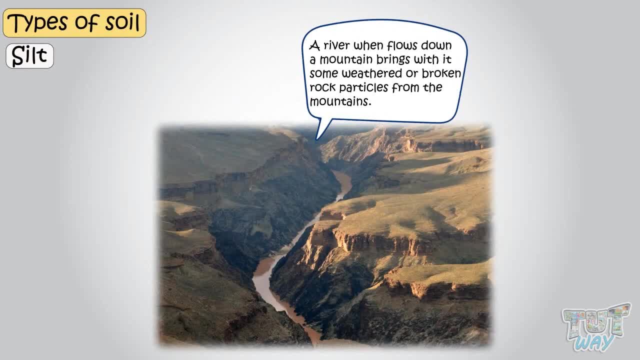 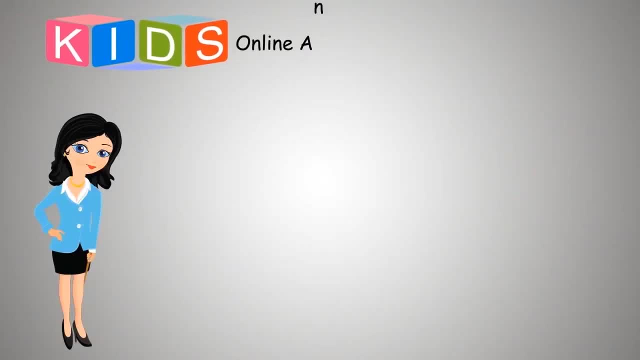 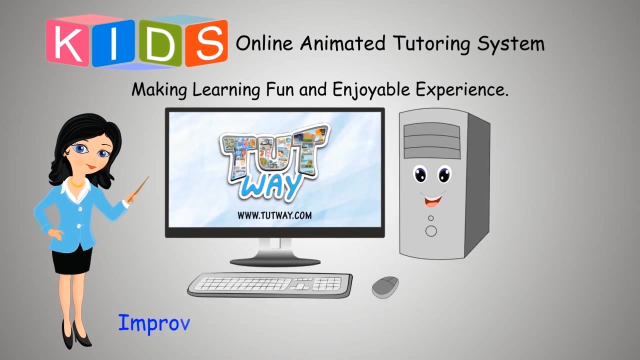 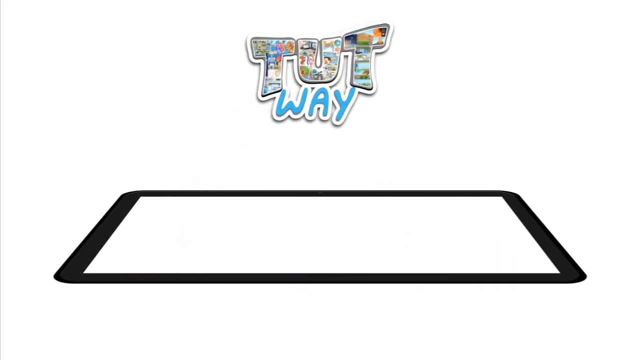 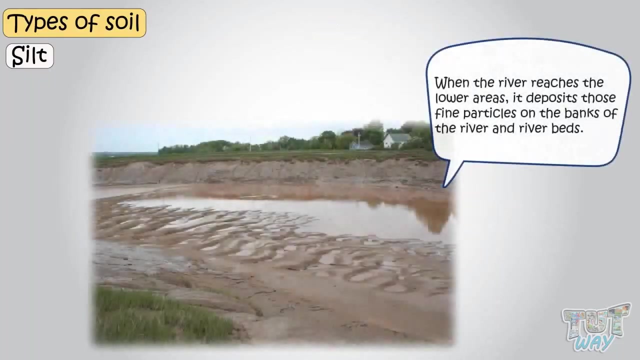 A river, when flows down a mountain, brings with it some weathered or broken rock particles from the mountains. TutWay has thousands of animated videos on math, English and science to clear the core basics of these subjects. When the river reaches lower areas, 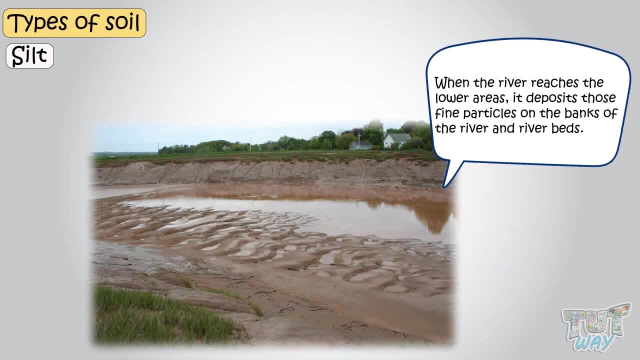 it deposits those fine particles on the banks of the river and riverbeds. It seems like very fine sand which is soft to touch, And this deposited sand is called silt. Now put some silt in a strainer and now pour water on it. 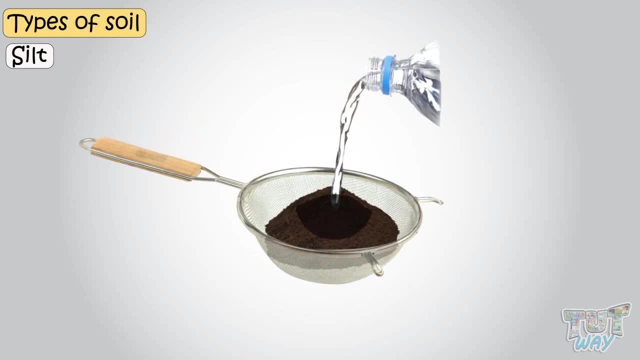 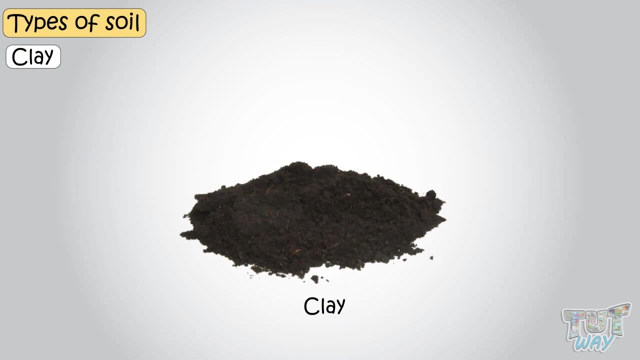 Water will drain through the silt slowly as compared to sand. So silt holds some water and water drains through silt slowly. then that through sand. Now we will learn about clay. Clay has the smallest rock particles among all types of soil. 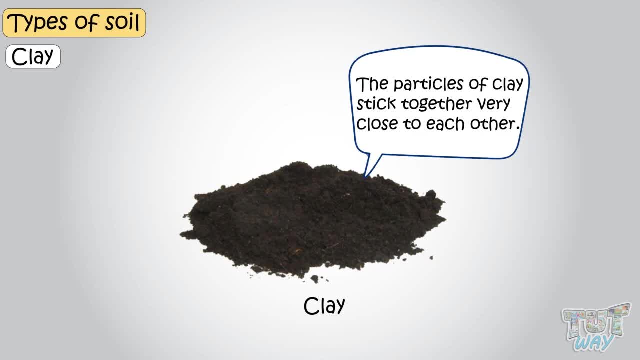 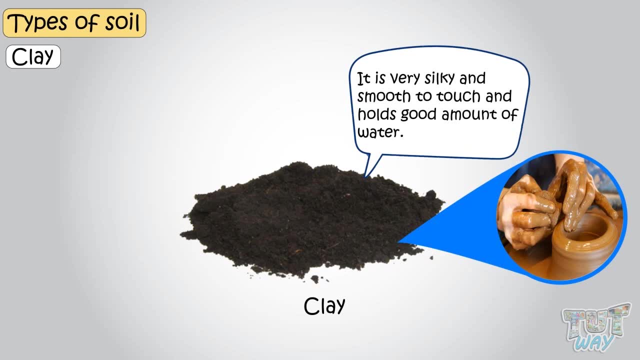 They stick together very close to each other. It is very silky and smooth to touch and holds good amount of water. That is, if you add water to clay, much of it will stay in the clay. Now take some clay in a strainer and now again pour water on it. 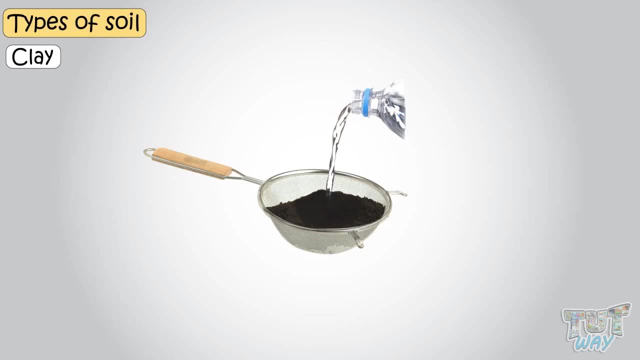 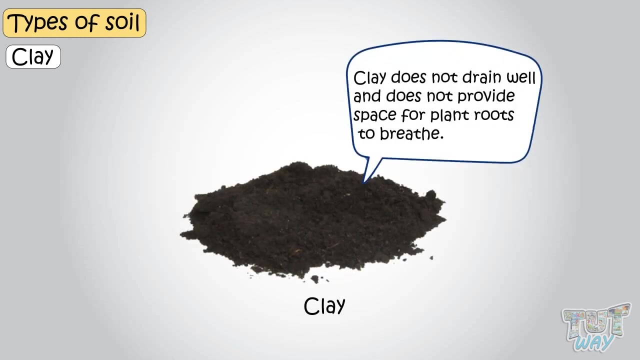 What do we see? Very little amount of water will drain through the soil, And that too, very slowly, Because clay holds the water and water drains through it very slowly. Clay does not drain well and does not provide space for plant roots to breathe. 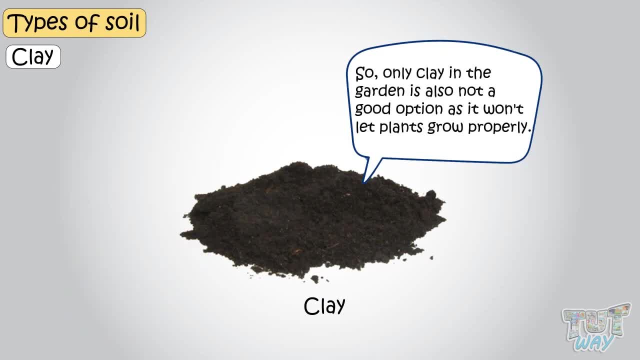 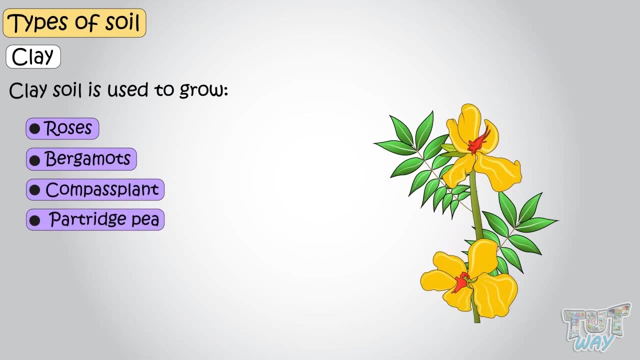 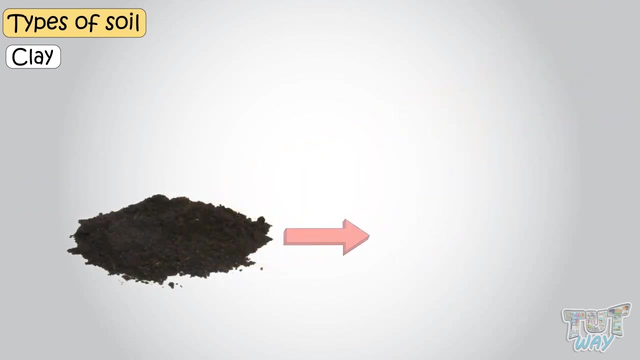 So only clay in the garden is also not a good option, as it won't let plants grow properly. Clay soil is used to grow roses, bergamots, compass plants and partridge peas. Clay can be fired or dried in the sun to make bricks. 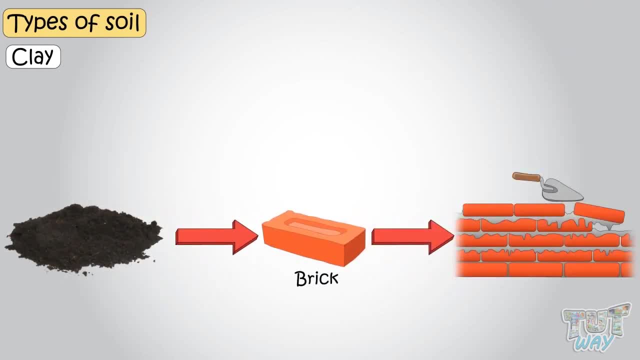 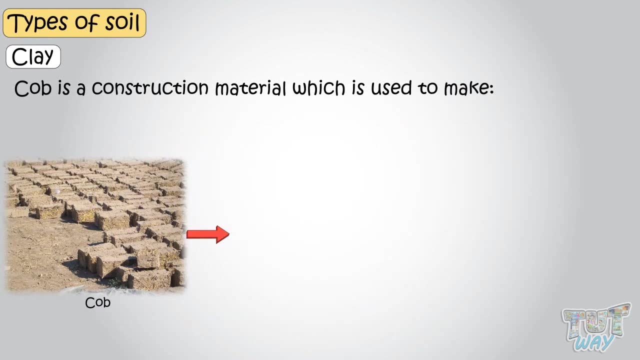 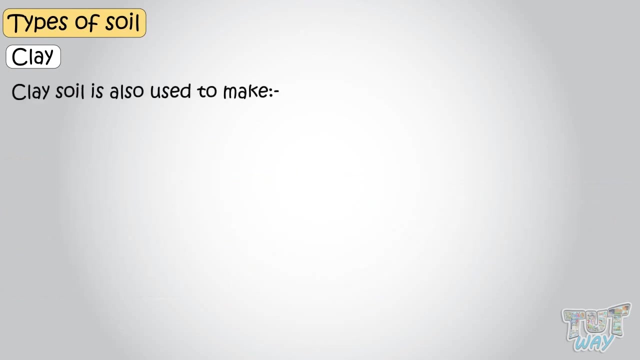 which are then used in construction of buildings. Clay combined with straw and sand makes cobb, And cobb is a construction material which is used to make buildings, ovens and benches. Clay soil is also used to make tools. Clay soil is also used to make tools. 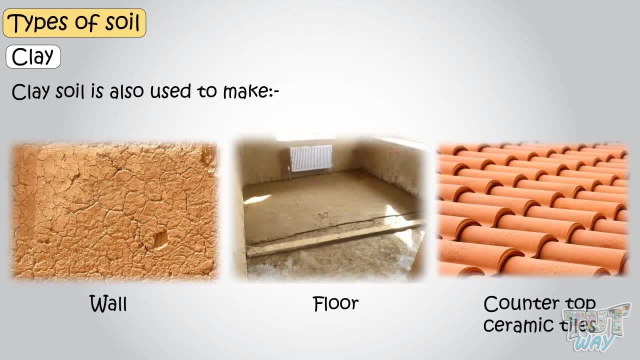 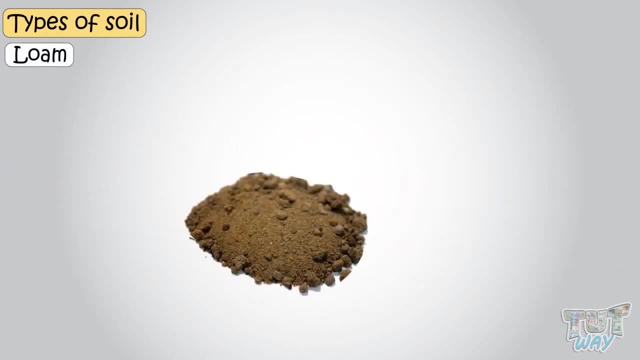 Clay soil is also used to make tools, walls, floors, countertop, ceramic tiles. Now here we have another type of soil, which is loam. Loam is a mixture of sand, silt and clay. The quality of loam soil depends on. 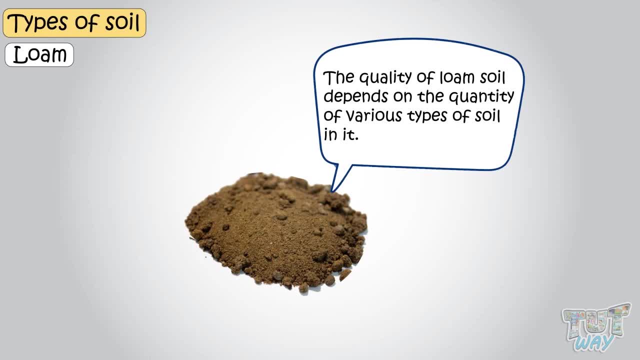 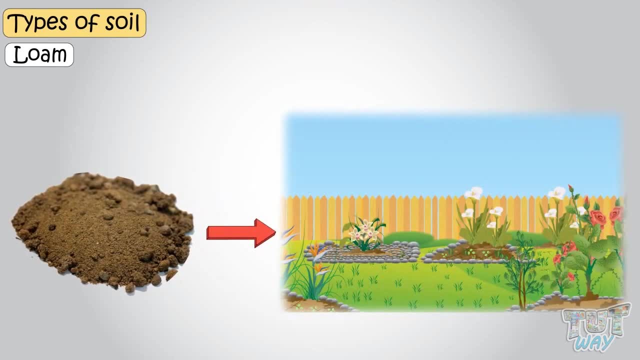 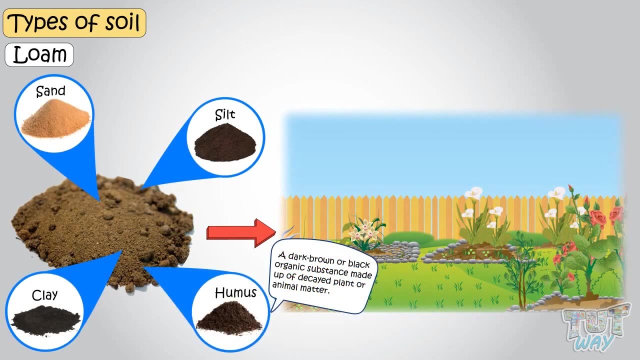 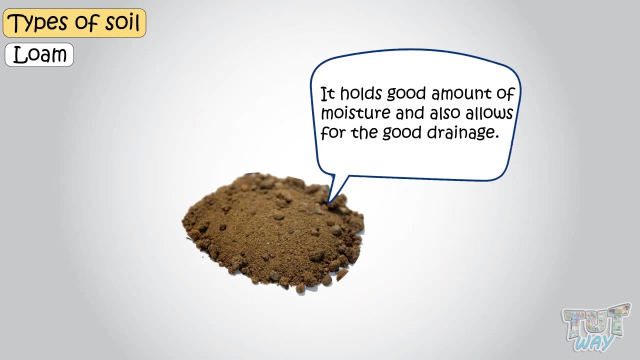 the quantity of various types of soil in it. This is why loam soil is always the first choice of a gardener, as it's best for plant growth, since it is a mixture of all types of soil and it has humus too, So it holds good amount of moisture and also allows good 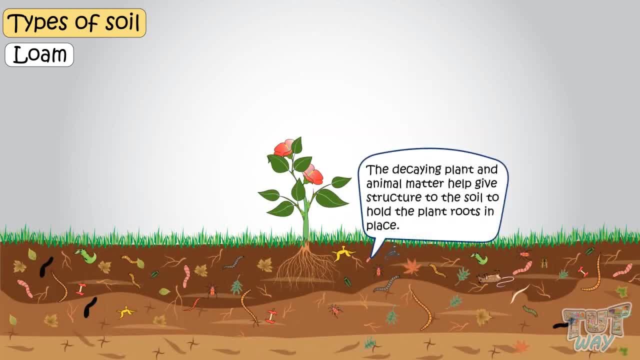 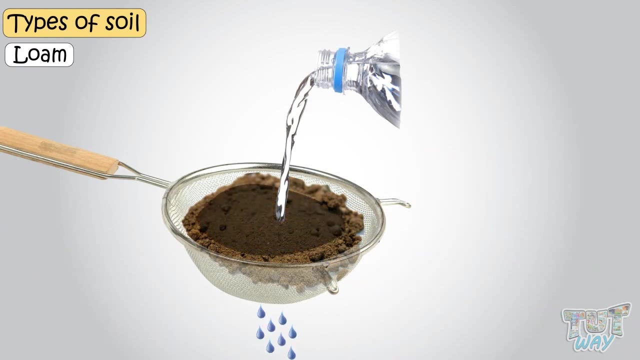 drainage. The decaying plant and animal matter help give structure to the soil to hold the plant roots in place. Loam Loam also holds just the right amount of water, neither too less nor too much. It lets some water in which, allowing the extra to drain. 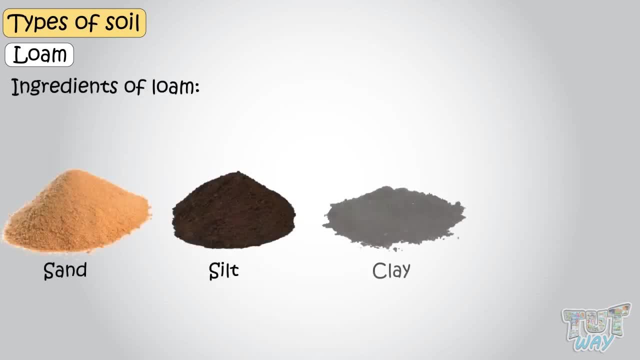 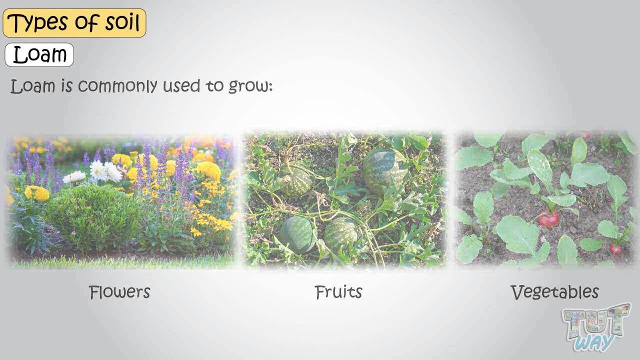 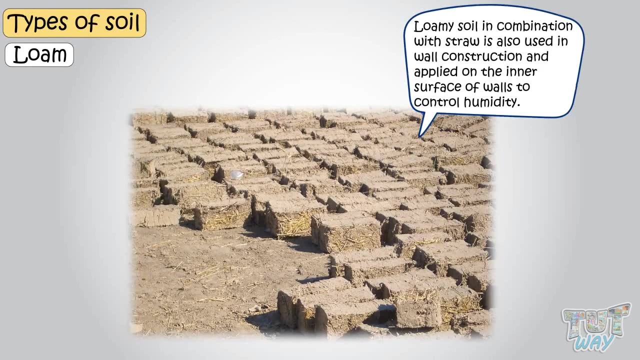 Ingredients of loam are sand, silt, clay and humus Loamy. soil is ideal for plant cultivation and is commonly used to grow flowers, fruits and a variety of vegetables. Seasoning Lily, Kitabu-, Baker & Ball. You will notice that Stella, a successor to 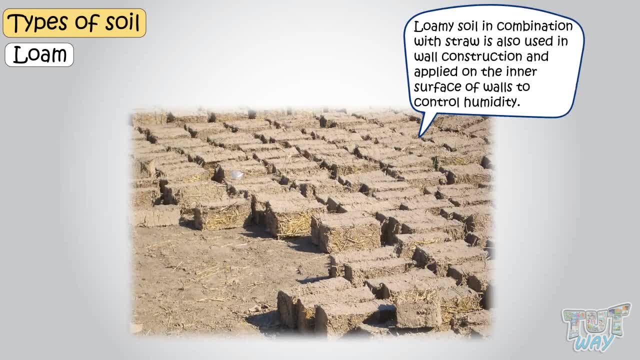 nahme was also used in structure that would have a lot of lightning overview. The soilblocks cover rich soil layer. Similarly, Loamy soil in combination with straw is also used in wall construction and applied on inner surface of walls to control humidity. Graeme Cyrontrygius: the best source and anticipative knowledge of soil structure. 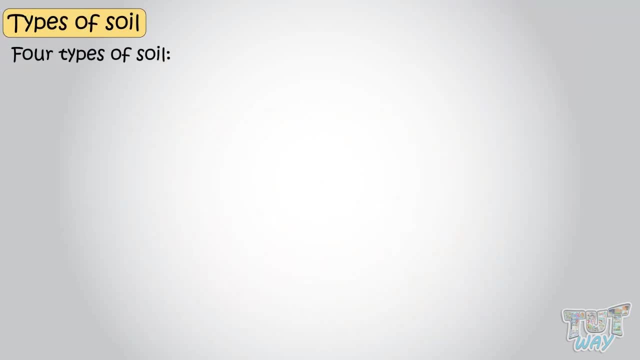 Now let's revise what we have learned about types of soils. We learned about 4 types of soil: sand, which has biggest rock particles. silt has particles of rock soaked into the soil. and silt has the highest amount of magnesium in it. Everyone.